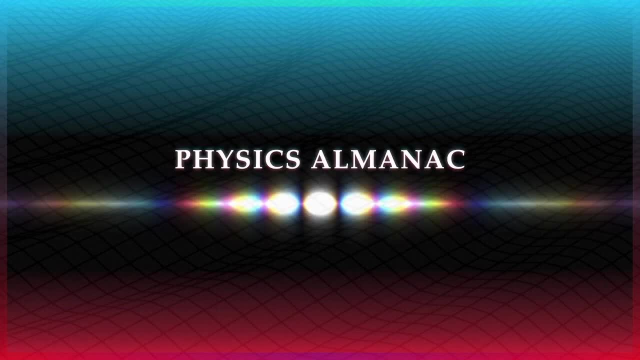 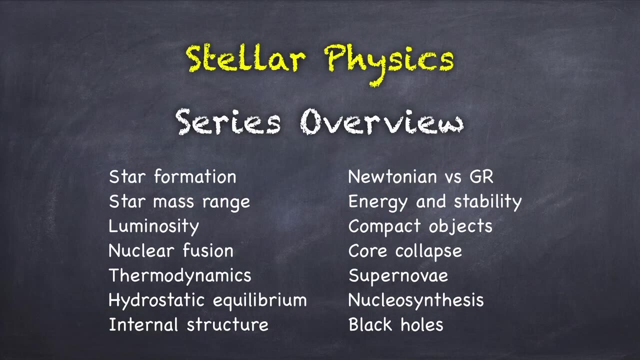 For more physics-related content, please subscribe. Welcome to the Physics Almanac. This is the first video in a series on stellar physics. Over the course of this series, we will cover, among other topics, star formation, star mass range, luminosity, nuclear fusion, thermodynamics as it pertains to stars, hydrostatic equilibrium, internal structure. 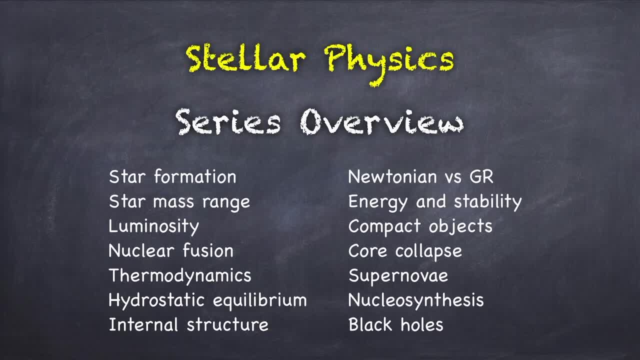 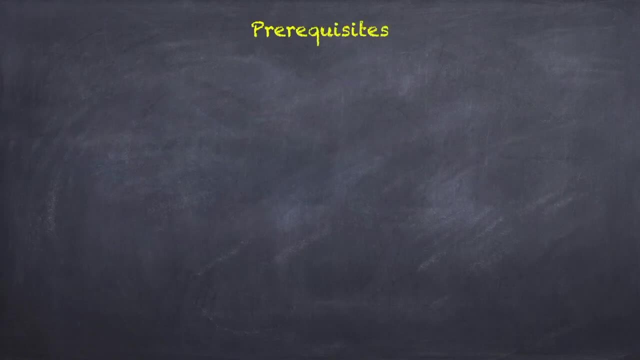 Newtonian stars versus stars in general, relativity, energy instability, compact objects, core collapse, supernovae, nucleosynthesis and black holes. Before we get started, we have to go over a few prerequisites In order to understand the material in this series. you will need a basic understanding of high school or intro college level physics. you'll need to be familiar with Newton's laws. 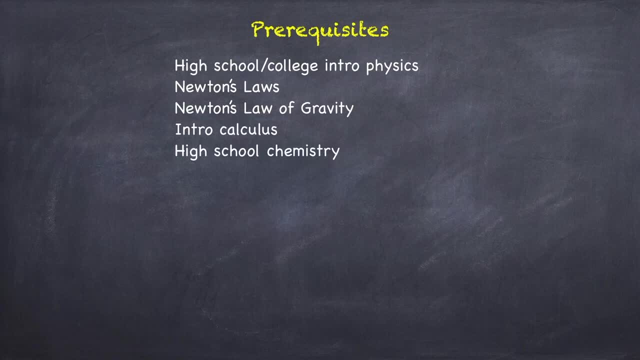 as well as Newton's law of gravitation. you'll have to have some understanding of calculus. at the very least, you'll need to know what a derivative and an integral are, and you'll have to have a basic high school chemistry level. 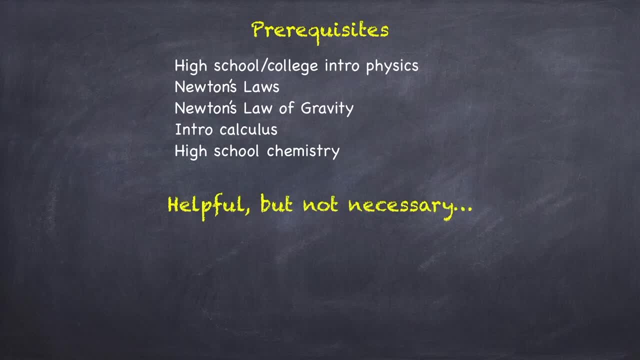 It would be helpful, but not necessary, if you also knew something about thermodynamics, quantum mechanics, general relativity and, in general. the more physics you know, the better. But if you don't know anything about these topics, we'll go over them as they come along. 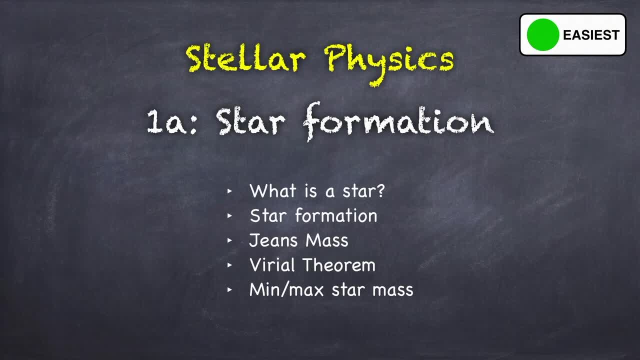 So in this first video we're going to go over star formation. We'll cover what a star is, how stars are formed, the gene's mass virial theorem and the minimum and maximum star masses. I've rated the physics level in this video as easiest. 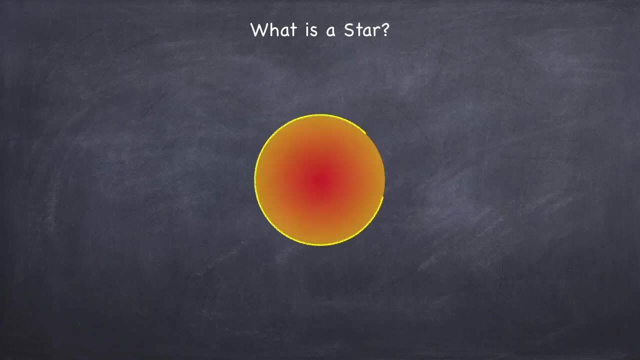 So what is a star? A star is a ball of gas, typically 75% hydrogen and 25% helium, that is held together by gravity At the center of the star. energy is released through nuclear fusion, which exerts an outward pressure counteracting gravity. 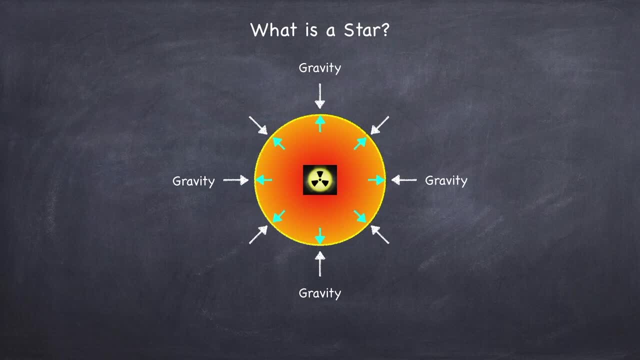 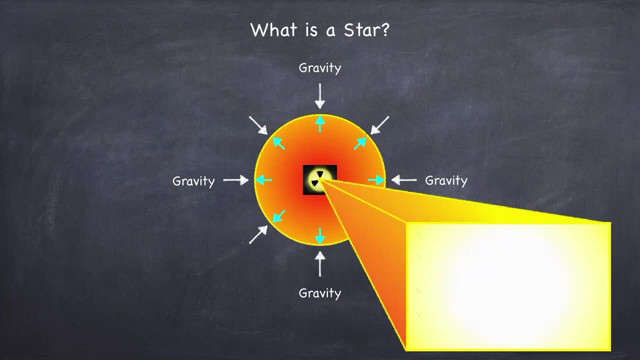 When the outward pressure balances the inward gravitational forces, we say that the star is in hydrostatic equilibrium. When I say that nuclear fusion takes place in the star, what I mean is four protons are turned into a helium nucleus. So here we have four protons which are just hydrogen nuclei. 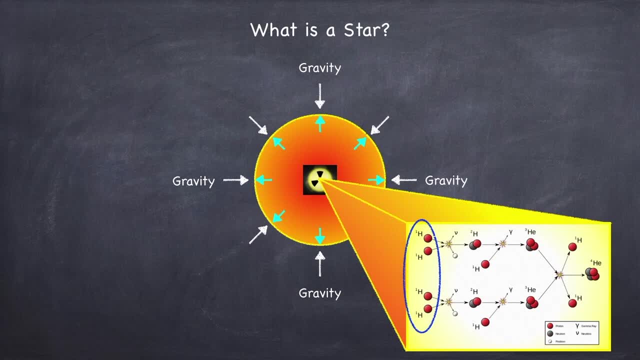 They're not hydrogen atoms, as the star is made up of a plasma, meaning that the electrons are not bound to the nuclei. So a plasma is basically just a sea of free nuclei and free electrons. So here we have the four protons which, through a chain reaction, come together and make one helium nucleus. 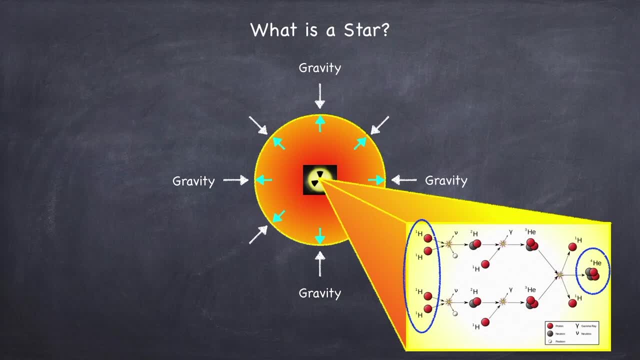 which is also called an alpha nucleus, So I might use those terms interchangeably. In the process, energy is released in the form of neutrinos and photons. The neutrinos don't really interact with anything and they just leave the star and they're basically a source of energy loss. 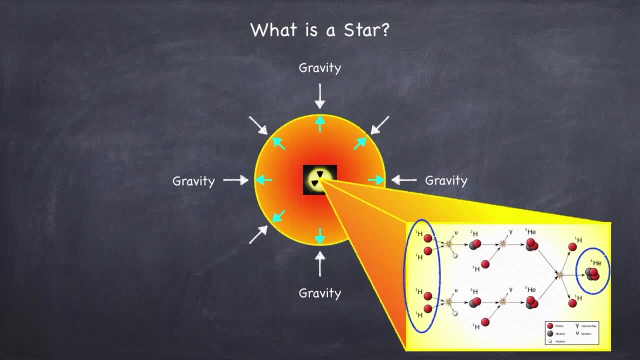 The energy in the photons is dumped into the star, and this is what heats the star up, causing the outward pressure that counteracts the gravitational inward collapse. In order for fusion to take place, you need a temperature of about 10 to the 7 Kelvin. 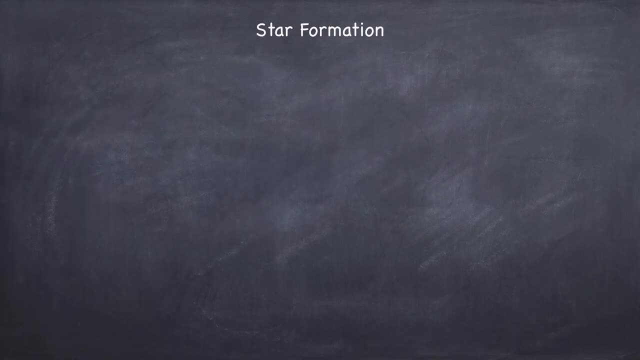 So how is a star formed? Let's imagine we have what's called a self-gravitating gas cloud. So this is just a cloud of gas that is loosely held together by gravity. So in this cloud, each particle is moving in an orbit from one side of the cloud to the other. 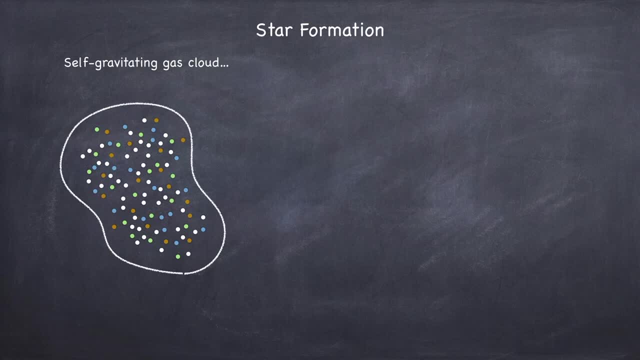 as a result of the gravitational pull of all the other particles. Now, at some point, something causes this cloud to collapse, And as it collapses it will heat up until it gets hot enough that nuclear fusion takes place and the star will turn on. 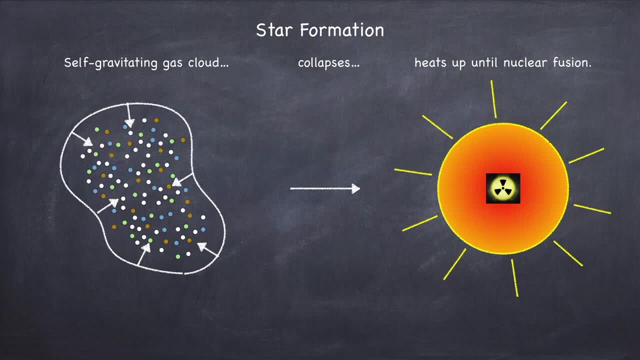 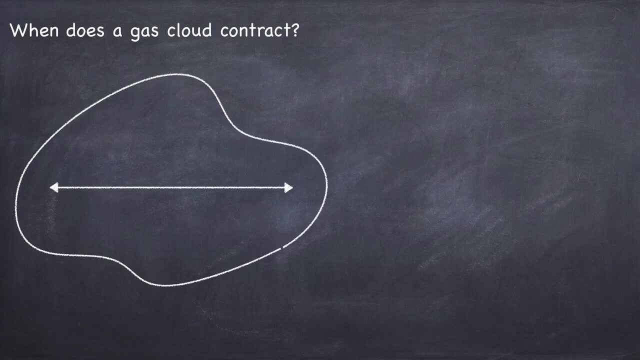 and it will cease to contract. Now the question is: when does a gas cloud collapse? So let's draw our gas cloud again and let's say it has a width L. Now let's say that on one side of the cloud. 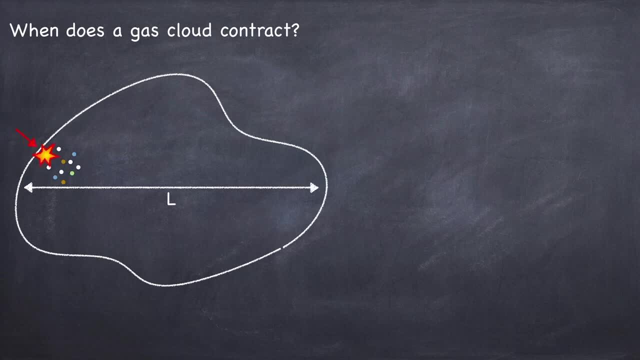 there's a bunch of particles and again they experience some disturbance. They will bump into the particles next to them, which will bump into the particles next to them, and this disturbance will propagate to the other side of the cloud. And the speed at which this disturbance propagates across the cloud. 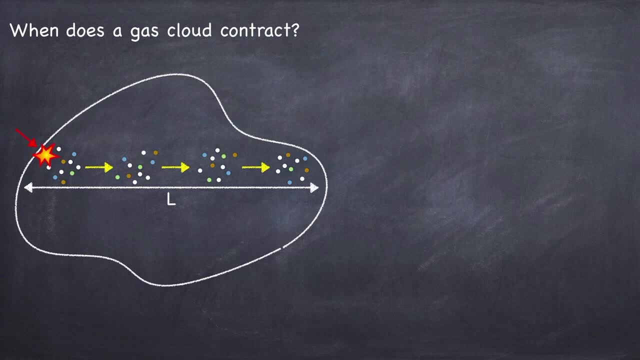 is the speed of sound, because that's what sound is: It's particles bumping into other particles. So this tells us how long it will take for the cloud to basically react, in a sense, or re-equilibrate, when the cloud collapses. 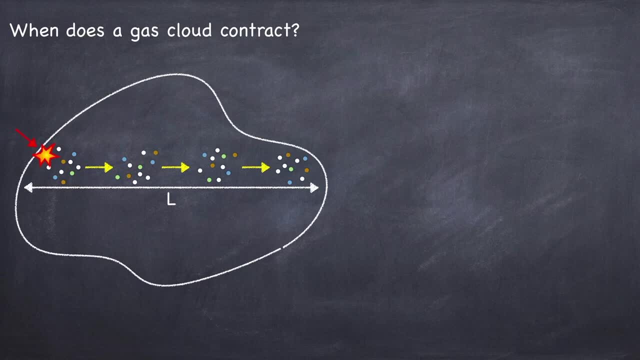 When a disturbance occurs. So the time it will take for this perturbation to propagate to the other side of the cloud is the sound crossing time, which is the width of the cloud divided by the speed of sound. So I'm calling here t sub s as the sound crossing time and c sub s is the speed of sound. 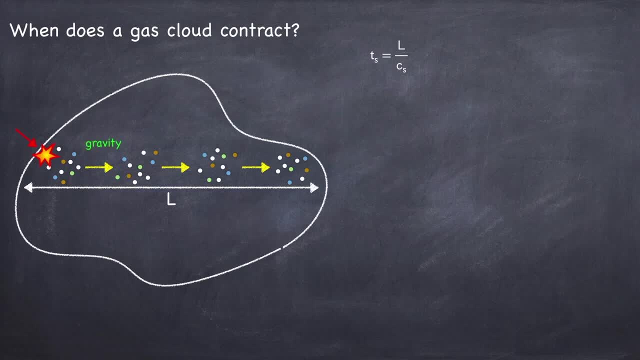 But there is gravity in this cloud, and so it may turn out that, due to gravity, particles will fall in faster than the speed of sound. If this happens in the time it would take for the cloud to react, the particles will fall in faster than the speed of sound. But if this happens in the time, it would take for the cloud to react. the particles will fall in faster than the speed of sound. But if this happens in the time it would take for the cloud to react. the particles will fall in faster than the speed of sound. 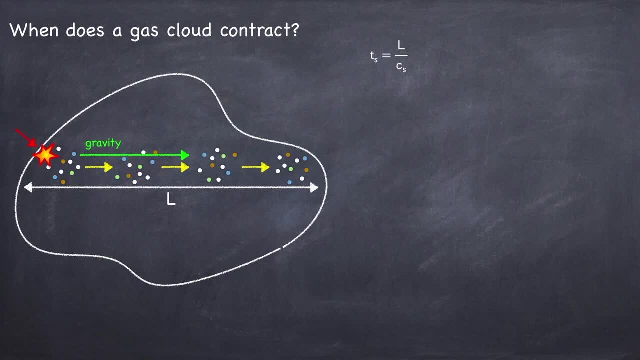 Due to the perturbation, the infalling particles will have reached the center of the cloud, So the cloud will go unstable. if the sound crossing time is greater than the freefall time, which I'm labeling here: t f f. The freefall time is the time it would take for an object to freefall. 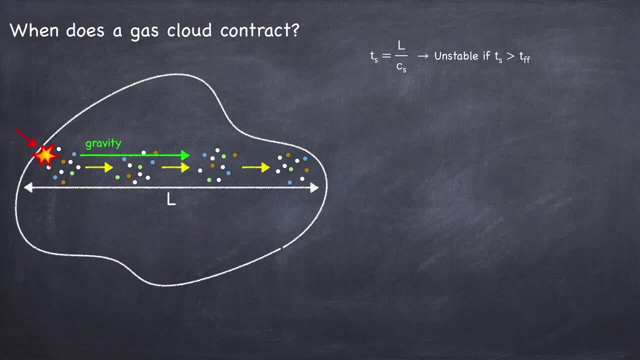 from the edge of the cloud all the way to the center. Now we have to solve for the freefall time, And we're going to do this with conservation of energy. So the energy here is just the kinetic energy, So which is one half times the mass. 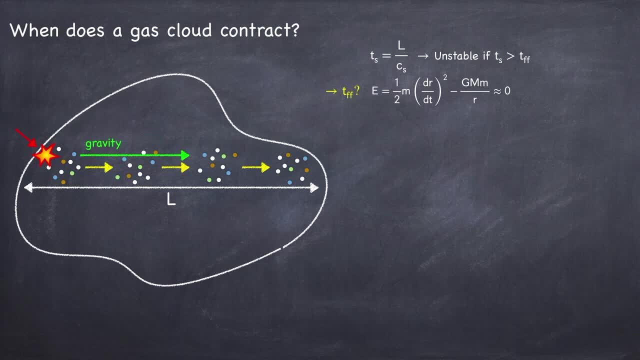 In this case, this little m is the mass of a particle or a blob of mass within this cloud, times its velocity squared, which is the derivative of position, minus the gravitational potential energy, which is going to be the mass of the cloud. 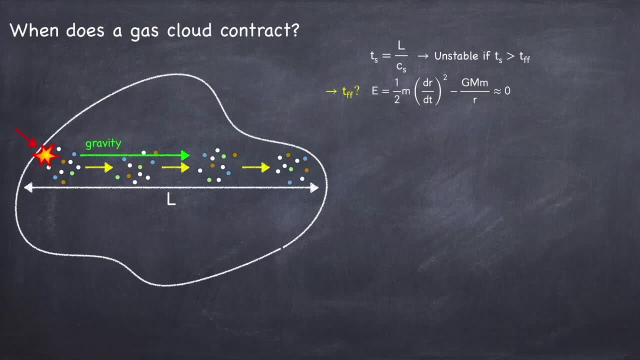 times the mass of this particle divided by its position, And since this cloud is very loosely bound, its energy is very close. We can cancel the mass of the particles and rearrange this to get a term for the velocity in terms of position. 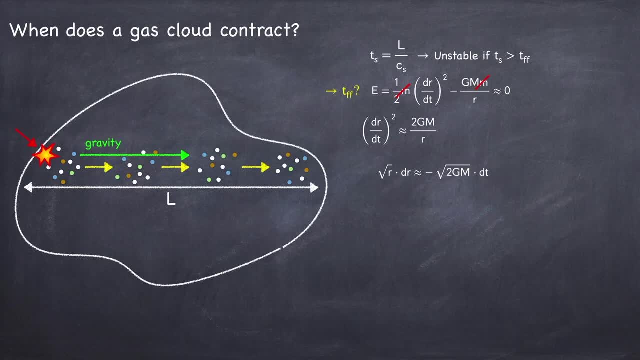 Now I'm going to bring all the r terms to one side and take the square root, And I've got a negative sign here to indicate that the material is infalling rather than outgoing. Now we integrate from the edge of the cloud to the center of the cloud in one freefall time. 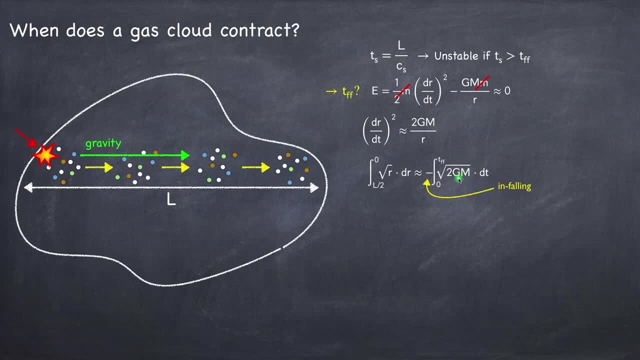 Keeping in mind here that this mass is falling in with the material. So this is the enclosed mass. Since it's falling in it's constant, It's always the same mass that's enclosed. This yields the following expression for the freefall time: 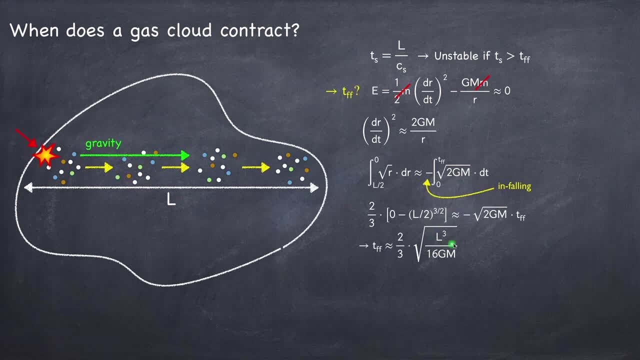 Now notice here that we have L cubed. Well, that's just the width cubed. So that's the volume of this cloud divided by its mass. So this whole term here is one over the density. So we can rewrite the freefall time as being: approximately one over the square root of Newton's constant times, the density. I'm ignoring the numerical factors here because they're approximately one, and anyways this is a fairly rough estimate. Now we set the sound crossing time to the freefall time and solve for L. 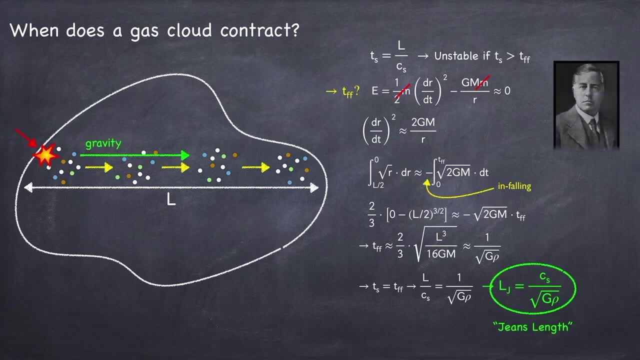 and we get what is called the Jeans Length, named after James Jyns. So we know that we got a frequency of L equal to zero with the gross mass of the cloud, So we not get to write C- Shepherd's time, which is one of the weights of what we can calculate. but this is still an acronym for PCR- WestwaysStephen's as well. This tells us that if a self-gravitating cloud becomes too extensively framment and we are able to break the R limit of the scale by managing r�, why we're doing that? 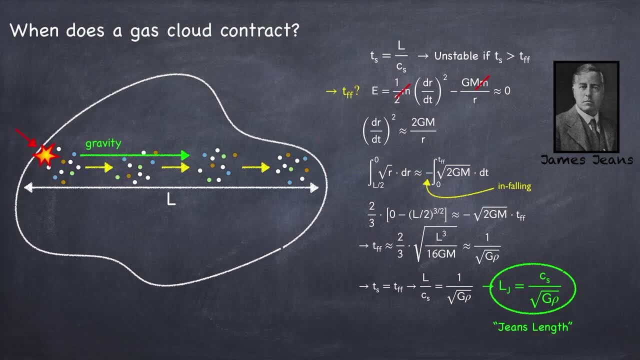 self-gravitating cloud becomes too extended, it will go unstable. We can also define what's called the gene's mass as the mass enclosed by a volume associated to the gene's length. So now we have a criteria for when a self-gravitating cloud will go unstable. 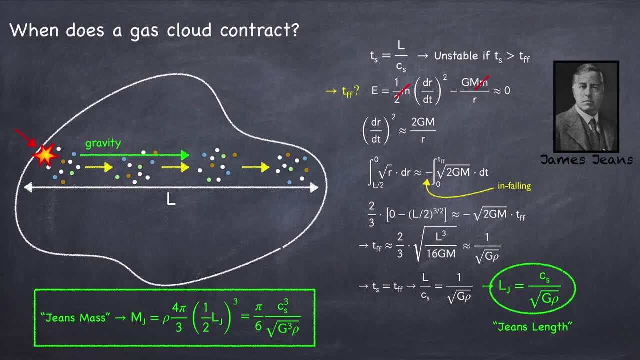 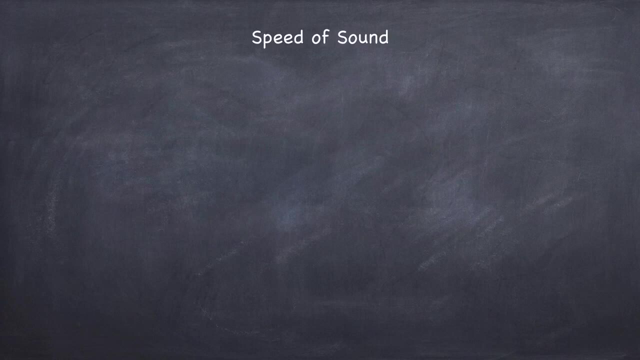 I should point out, though, that this doesn't mean it will collapse. It could go unstable and expand, in which case it will just disassociate. Now let's take a look at the speed of sound. The speed of sound squared is given as the partial derivative of pressure, with 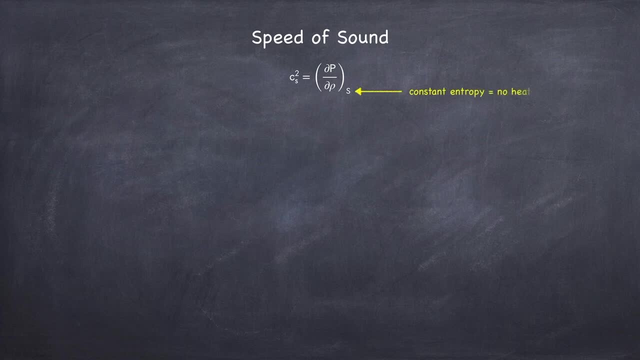 respect to density at constant entropy. Capital S here is entropy, So constant entropy is just another way of saying no heat flow. For the purpose of this video. I'm going to show you how to use the speed of sound to get the temperature. 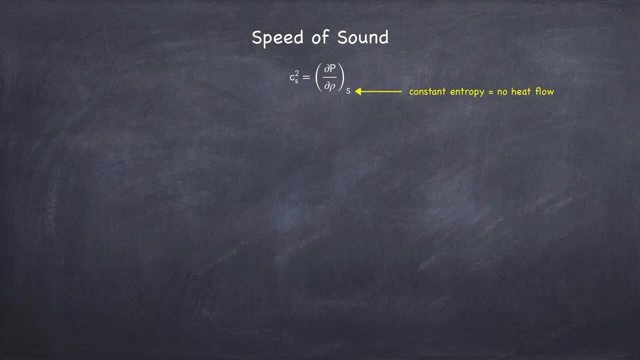 I'm not going to derive this equation, we're just going to take it as a given. Now, in the case of an ideal Boltzmann gas, you may recall from your high school physics that we have the ideal gas law and a relationship between the average. 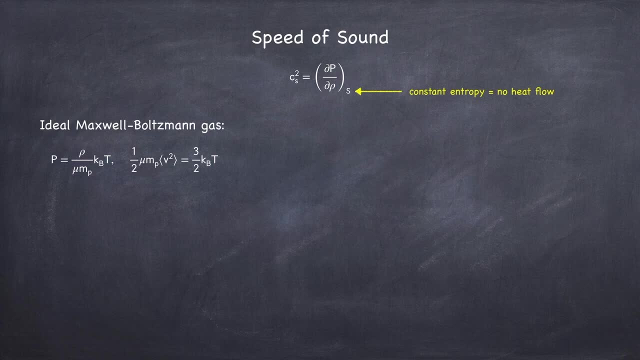 particle velocity and the temperature. You may know the ideal gas law, as PV equals nkt, I've simply written n over v and it's written as rho divided by the average particle mass, So Rho divided by the average particle mass, So Rho divided by the average particle mass. 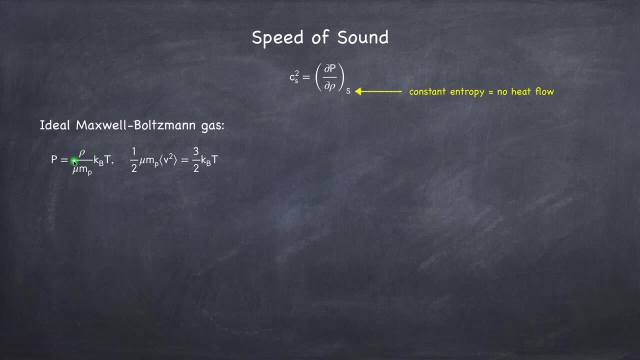 rho divided by the average particle mass is just the number of particles divided by the volume, And this quantity, mu, here is defined as the average particle mass in units of a proton mass, which I've called m sub p. In the case of an adiabatic process, which is 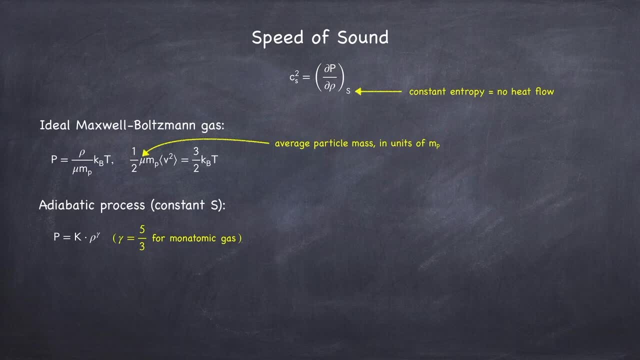 just another way of saying constant entropy or no heat flow. the pressure will be equal to a constant k times the density raised to another constant gamma Gamma is called the adiabatic index and in the case of a monatomic gas is 5 thirds. Now we can take these three. 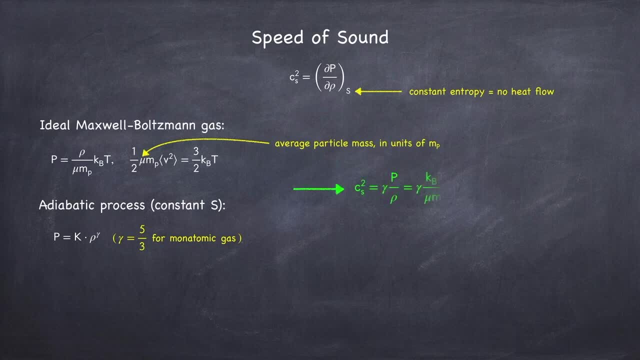 equations and plug them into our expression for the speed of sound, and we find that the speed of sound is approximately the average particle speed or, more specifically, the root mean squared velocity. If you're enjoying this video so far, please like and subscribe, and hit the bell icon. 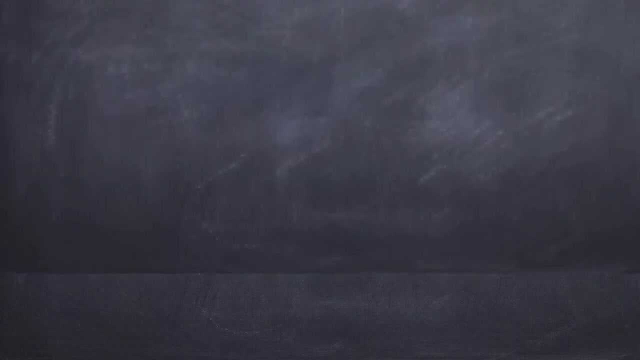 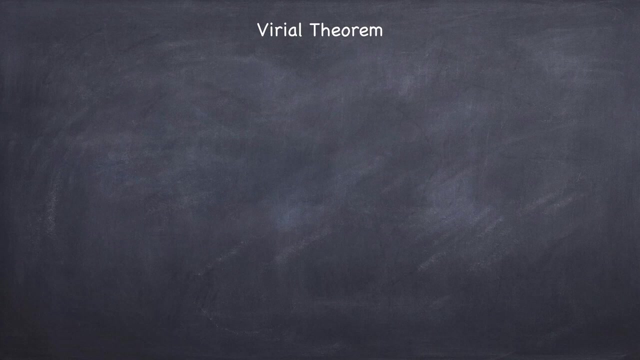 Now we're going to go over the Virial Theorem. This is a very important theorem in astronomy as it's used very often, but I'm not going to derive it because it's a pretty long derivation and the whole thing is on Wikipedia, if you're interested. Plus, we're not sure that this 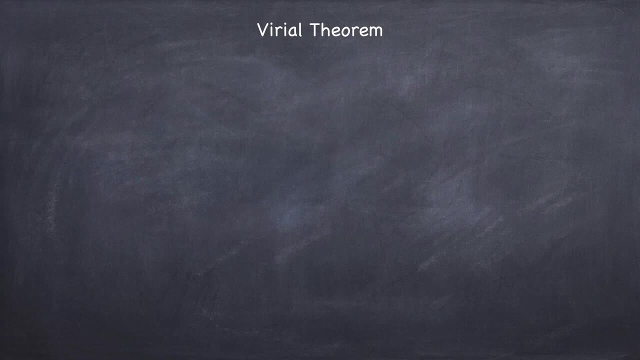 theorem actually holds. There are good reasons to think it probably holds, or, at the very least, that it's approximately true. The theorem is a very important theorem and it's a very important one. The theorem states that if you have a system with total kinetic energy Ke bound by a 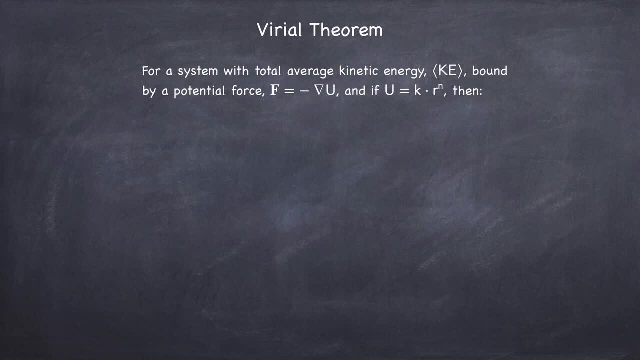 potential force, which is just a force that can be written as the negative gradient of a potential, which I've called U here. and if the potential is of the form, a constant times position to the n, where n is a number, then the kinetic energy is equal to n over. 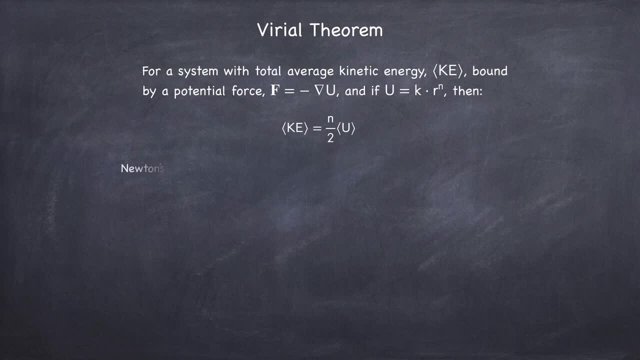 2 times the potential energy. In the case of Newton's law of gravitation, the potential energy between two particles, which I'm labeling i and j, is given as the negative of Newton's constant times, the product of the masses divided by the distance between them, which I'm calling 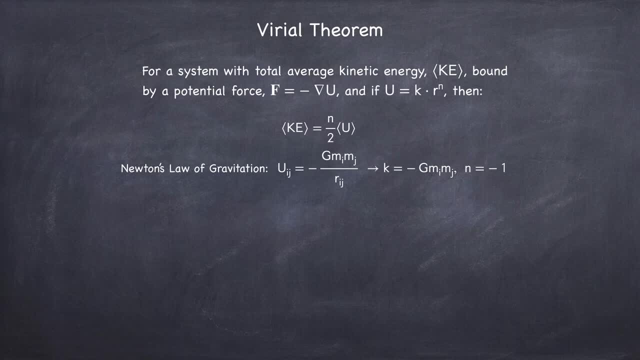 r sub ij. Matching this to our expression for U, we find that K equals negative, G times the product of the masses and n equals negative 1. The total potential energy will be the sum of the potential energies between each particle. So if you have a system with total 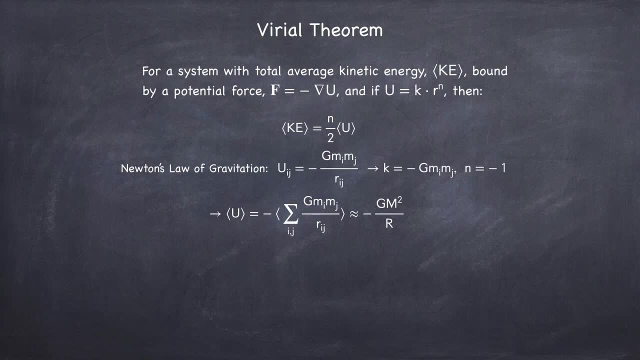 energy. you can write down the kinetic energy in terms of the potential energy. and you can write down the kinetic energy in terms of the potential energy, And this will be approximately equal to negative G times the mass of the cloud squared divided by its radius. In reality, there's going to be a numerical factor in front of this determined. 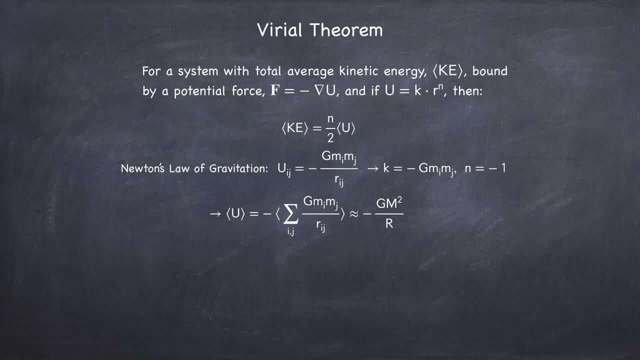 by how the mass is distributed in the cloud, but it's typically of order 1, usually something like 3 fifths or 1 half or somewhere around there. So I'm just going to say it's approximately 1.. The Virial Theorem now allows us to write down the kinetic energy in terms of the potential. 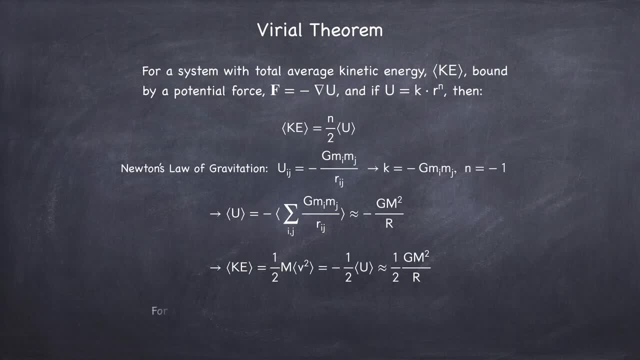 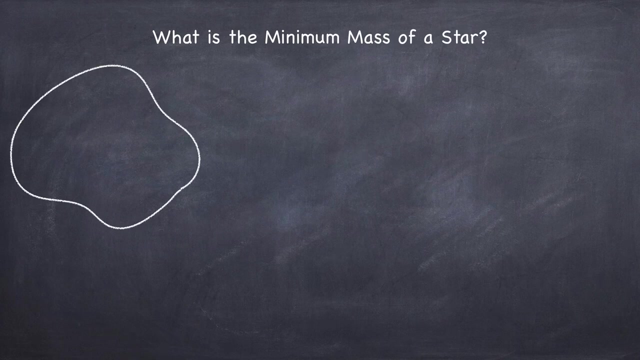 energy and in the case of a single particle, we can relate its average kinetic energy to its average potential energy by simply replacing one of the masses with the mass of that particle. Now let's discuss what is the minimum mass a star can have. We have a collapsing cloud. 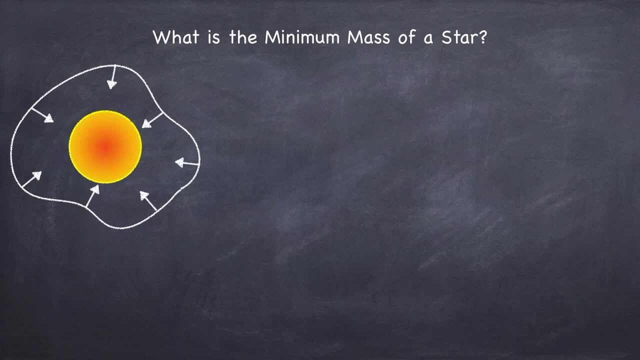 of gas that heats up and eventually will get hot enough for nuclear fusion to take place. It turns out that the lower limit on a stellar mass is determined by quantum mechanics. At some point, if this cloud continues to contract, it will become so dense that the average electron 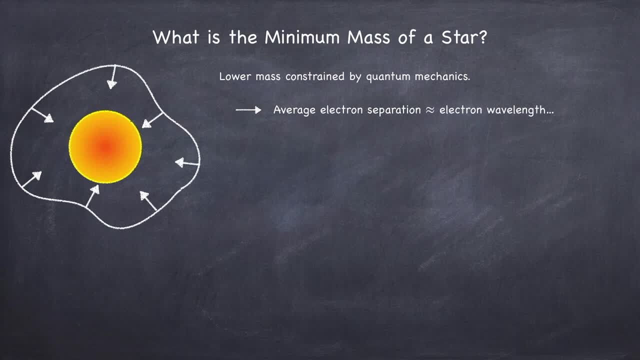 separation will be approximately the same as the electron wavelength. If you don't know, in quantum mechanics every particle has a wavelength that is associated to its momentum, And if a cloud ever gets to such a regime, classical mechanics will no longer hold, as 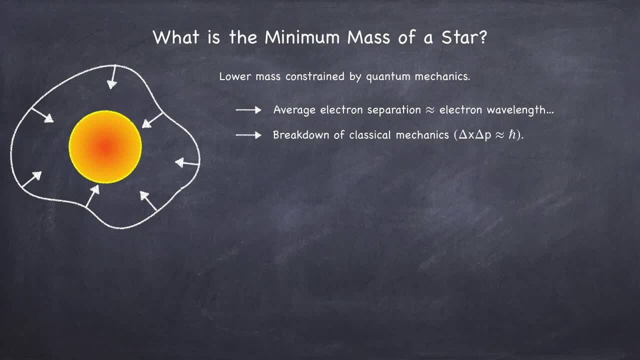 we will be pushing the limits of the Heisenberg uncertainty principle, which says that the uncertainty in the position times the other side is equal to the density of the particle. Now, in this case, since we'll be at that limit, delta x times delta p will be approximately. 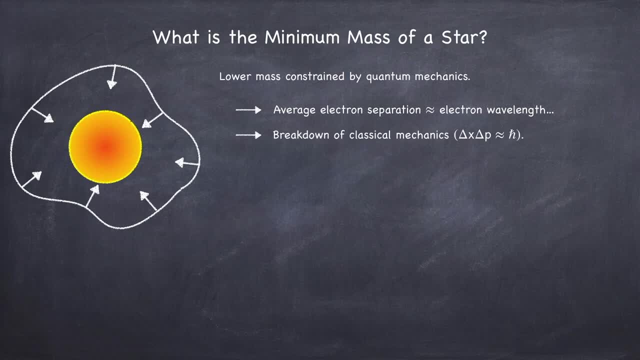 h-bar. It turns out that in this regime, the temperature will cease to increase with density. Right now, we're just going to take this as a fact, but we will eventually derive this when we talk about compact objects, Since the temperature will no longer increase with density. it doesn't 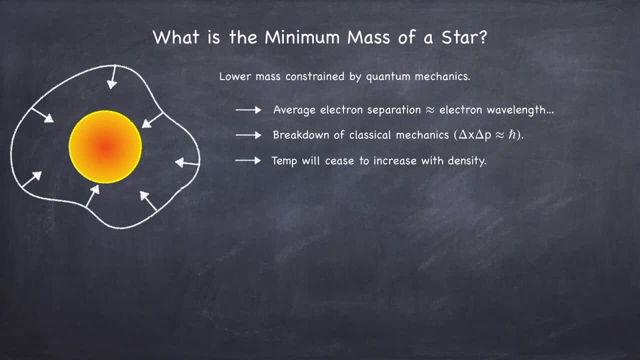 matter if this cloud continues to contract at this point. If it's not hot enough for fusion to take place, it will never be hot enough for fusion to take place. So this is how we're going to find the minimum mass of a star. Now let's write down the 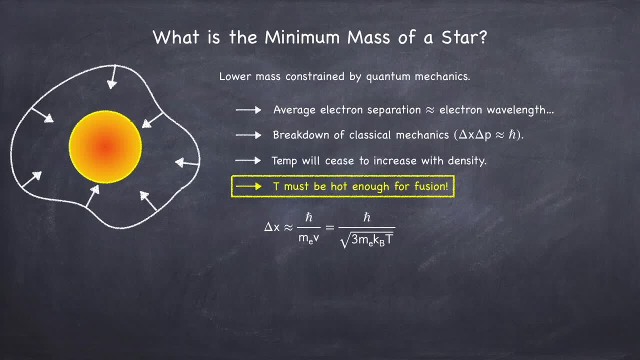 average particle separation as h-bar divided by the momentum of an electron, which is just its mass times its velocity, And this can be rewritten in terms of temperature by using the fact that the kinetic energy is related to the temperature. Now the density will. 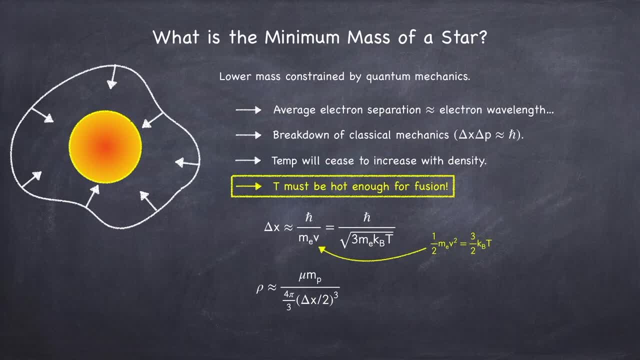 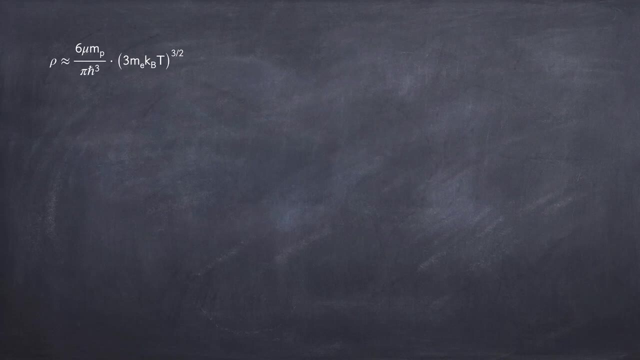 just be the average particle mass divided by a volume associated to this separation: delta x. So now we have an expression for the density in terms of temperature. Let's continue this on another board. I'm going to write down the expression we just found for density in terms of temperature. Now we're going to use the Virial Theorem to relate. 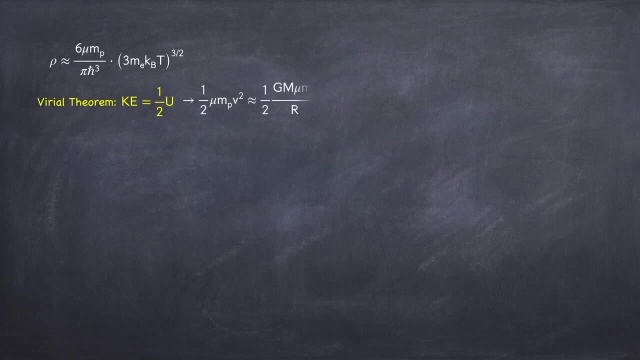 the kinetic energy to the potential energy. Again, I can replace the kinetic energy with the temperature And I'm going to use the fact that the volume is simply the mass divided by the density to replace r. This gives us the following expression for the temperature in terms of: 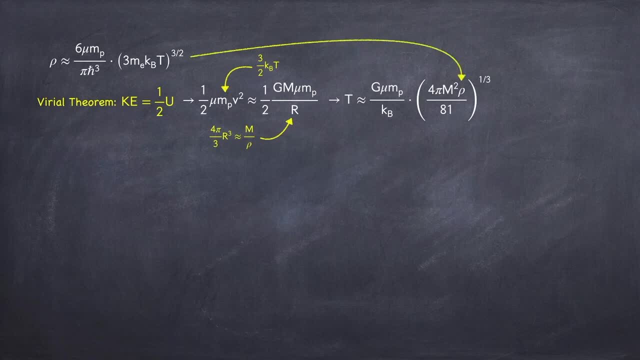 the density and the mass. We now can substitute our original expression for the density into this equation and solve for temperature, And we find that the temperature is proportional to the mass, to the 4 thirds. We can now plug in all the numbers. Mu for a star is typically: 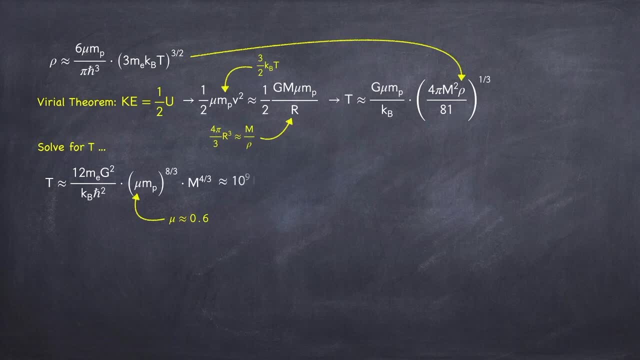 around 0.6. Or 0.7. And we find that the temperature is about a billion degrees Kelvin times the mass to the 4 thirds in units of solar masses. So this symbol here, a circle with a dot in it, is a symbol used in astronomy to represent the Sun. So this is just mass divided by one. 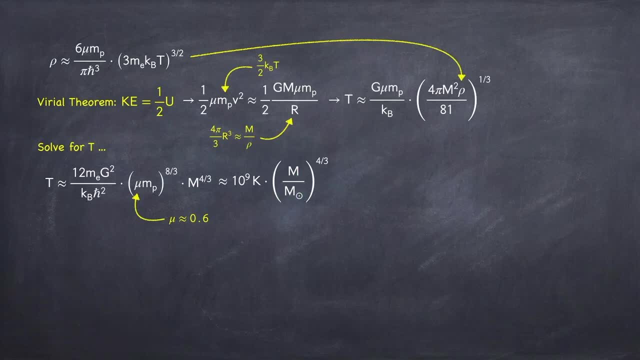 solar mass. That's what this means here. Now, we said earlier in this video that in order for fusion to take place, the temperature must be greater than 10 to the 7 Kelvin. Now, here we have the maximum mass, So we can solve for mass And we find that the minimum. 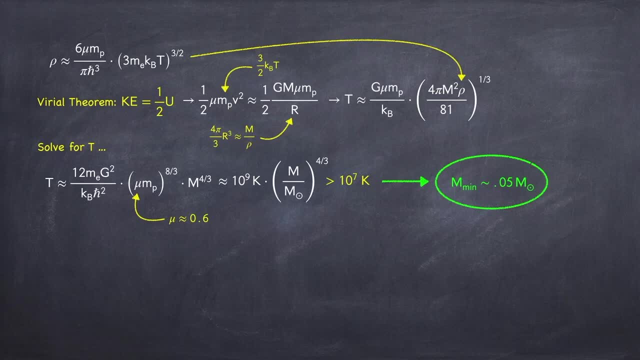 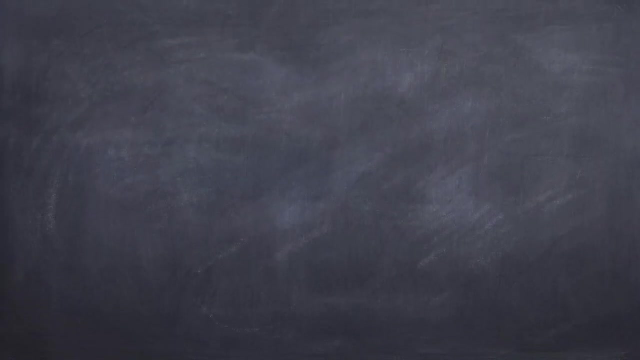 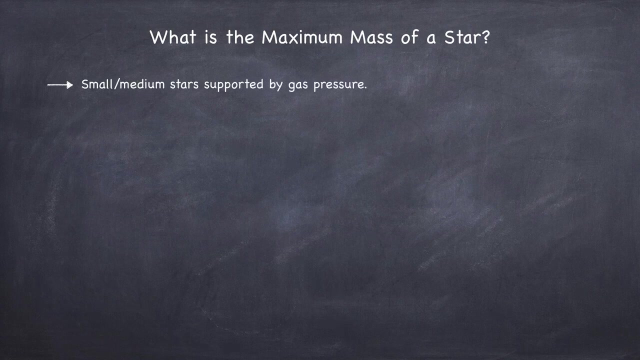 mass is about 0.5 solar masses. This is a theoretical limit, But it should be noted that the smallest observed star that I know of is about a tenth of the solar mass, So that agrees pretty well with this theoretical limit. How about the maximum mass of a star? So for typical stars, they are supported by gas pressure. 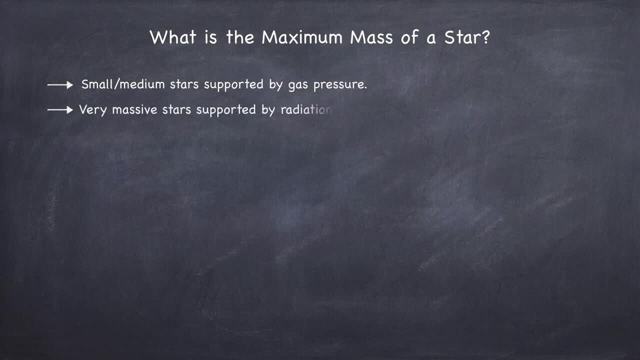 if stars get really massive, they end up being supported by radiation pressure. And when a star is supported by radiation pressure, they can go unstable due to general relativity. So the upper mass limit will be determined by what's called the general relativistic instability. So in order to 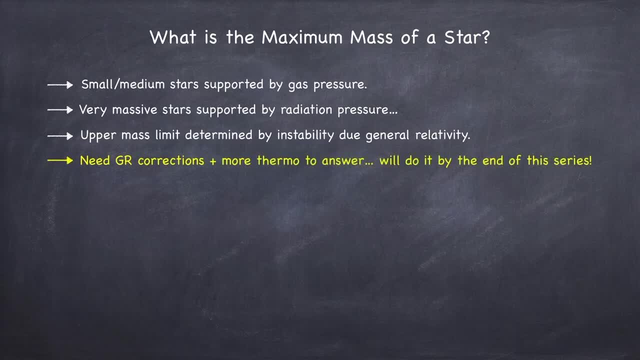 find the maximum mass, we're going to need to know something about general relativity, as well as a better understanding of thermodynamics. So we won't be able to do it in this video, but we will by the end of this series. 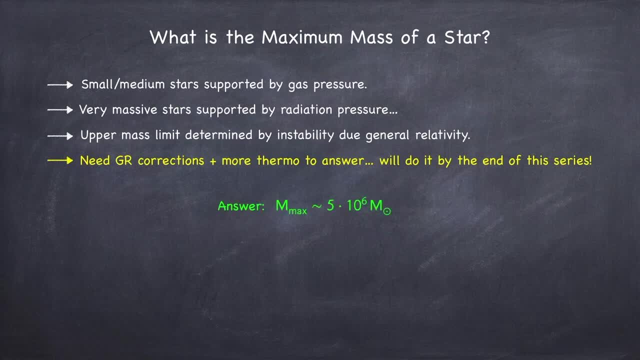 For the meantime, I'll just tell you that the maximum mass is about 5 million solar masses. It should be noted that this is again just a theoretical limit and that the largest star observed that I know of is about 250 solar masses. So 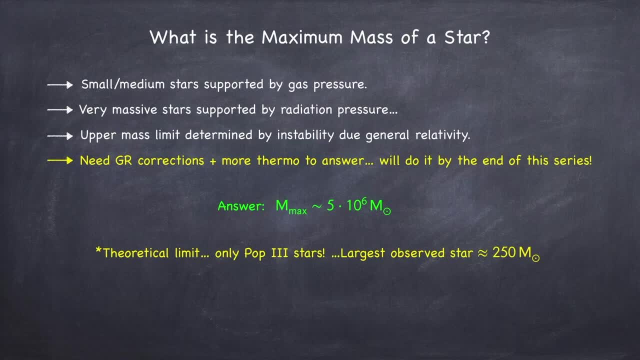 nowhere near this 5 million solar mass limit. It's also important to know that such a large star could only exist in what are called POP3D. POP3 stars is a term astronomers use when referring to the first generation of stars in the universe. So a while back, astronomers. 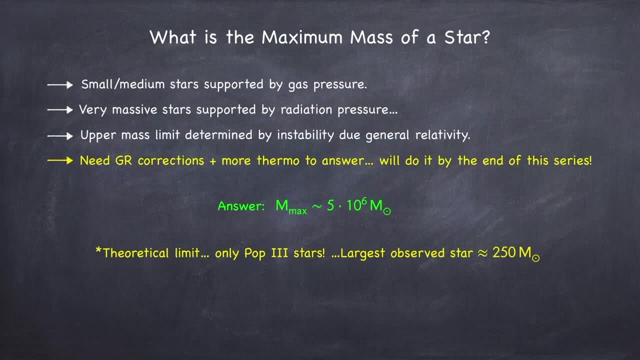 categorized stars into three generations: POP1 stars, which is the generation of stars that are around today. POP2 stars, which is the generation before that. and POP3 stars, which is the first generation of stars. This categorization of generations of stars is not really used today that much. 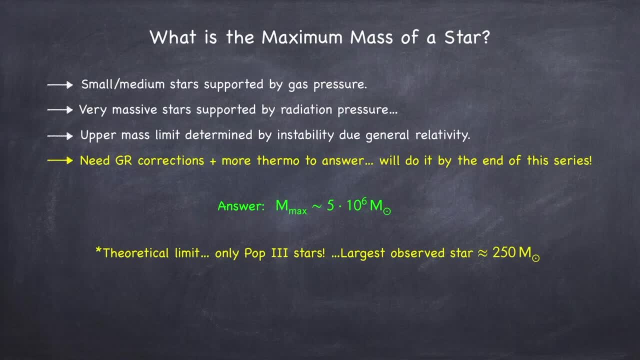 However, for sure, there once was the first generation of stars, and so those are still called POP3 stars. Now, what's special about those stars is that they're made up of what's called primordial abundances. They have no heavy metals in them. They're entirely helium and hydrogen and maybe a tiny bit of. 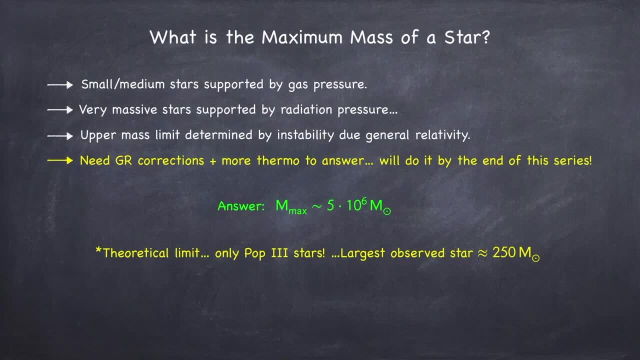 lithium, And by heavy metals here I just mean anything above helium. When a star has heavy metals in it, they act as catalysts and increase the nuclear production rate. So if you ever had such a massive star with heavy metals in it, it would just explode.